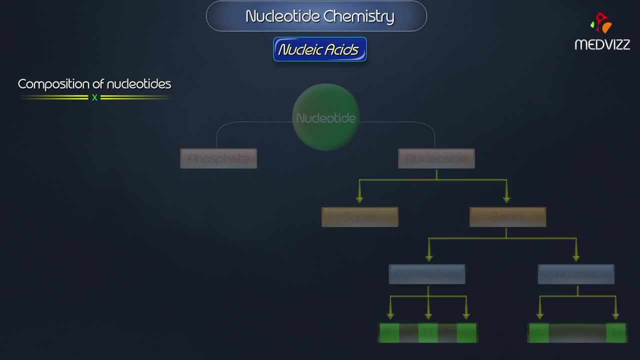 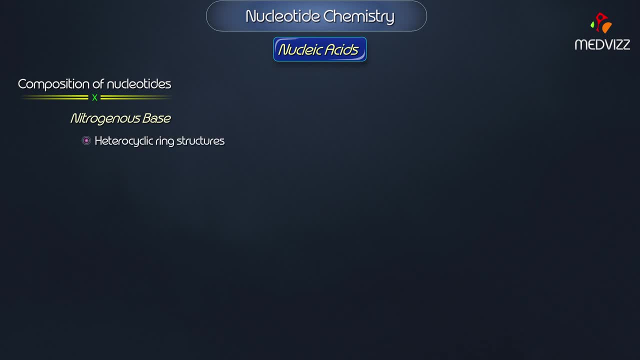 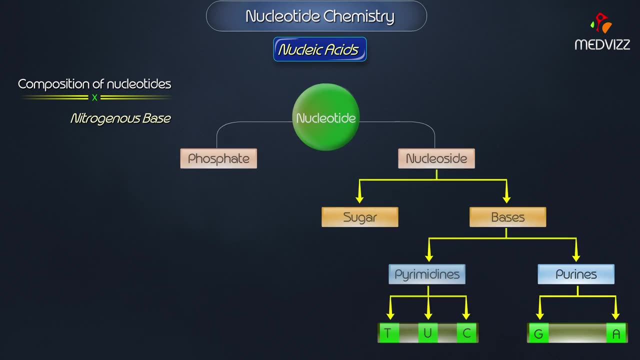 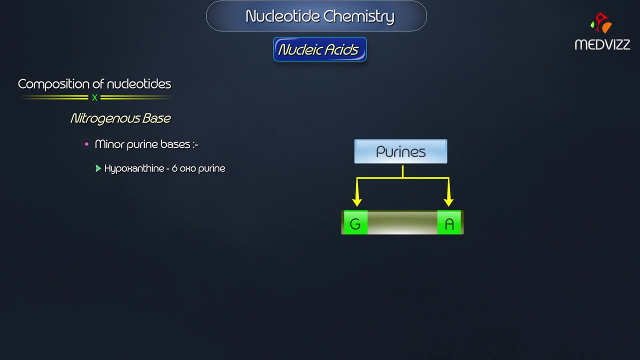 Nitrogenous Base. Nitrogenous Base are nitrogen-containing heterocyclic ring structures. Two types of nitrogenous bases are purine and pyrimidine. Purine bases are adenine and guanine. Minor purine bases are hypoxanthine-6-oxopurine, xanthine-2,6-dioxopurine, uric acid-2,6,8-trioxopurine. 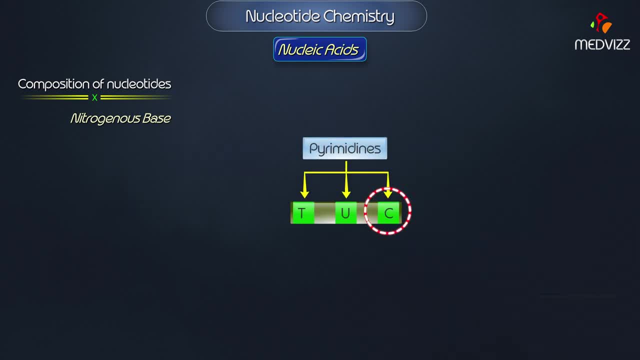 Pyrimidine bases are xanthine-2,6-dioxopurine uric acid-2,6,8-trioxopurine Pyrimidine bases are cytosine, uracil and thiamine. 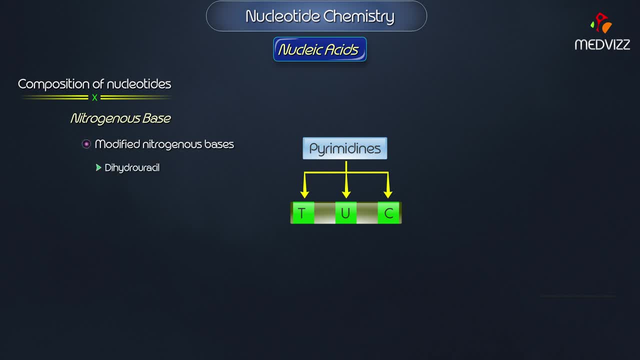 Modified nitrogenous bases are: dihydrouracil, pseudouridine, 5-methylcytosine, dimethylaminoadenine, 7-methylguanine. Important Points: Cytosine is present in both DNA and RNA. 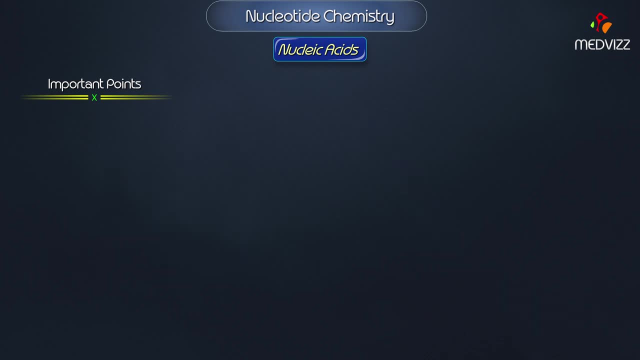 Uracil is present only in RNA. Thiamine is present only in the DNA. Most common modified bases are methylated forms of major bases, Pentose sugar. There are two types of pentose sugar: D-ribose sugar in RNA to deoxy-D-ribose sugar in DNA. 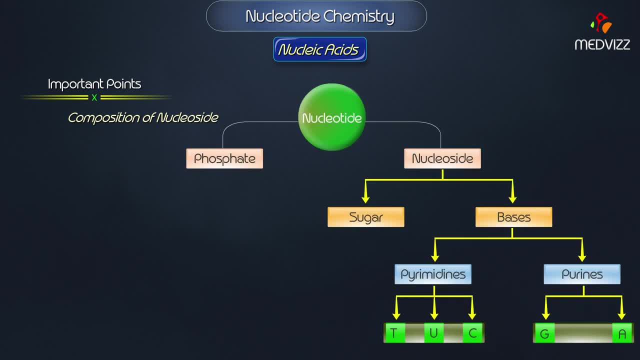 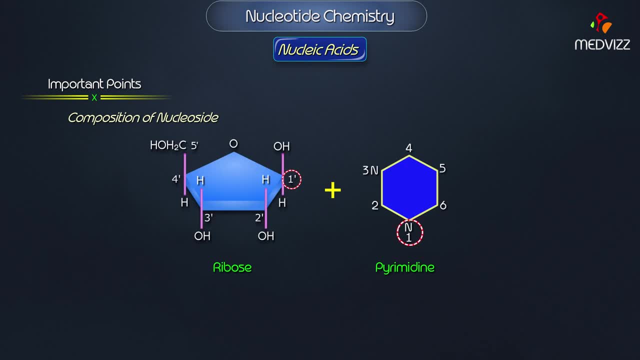 Composition of nucleoside. It is made up of a nitrogenous base plus pentose sugar, C-1 of ribose or deoxy-ribose sugar, joined covalently to N-1 of pyrimidine or N-9 of purine. 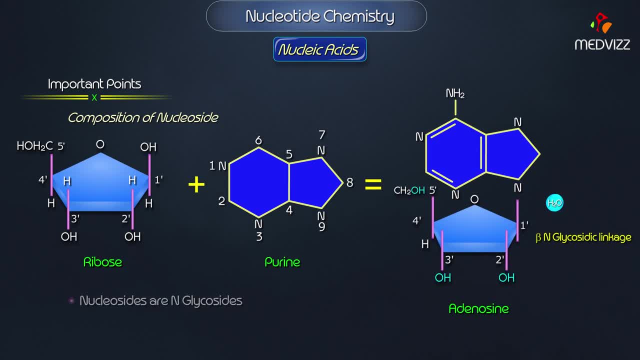 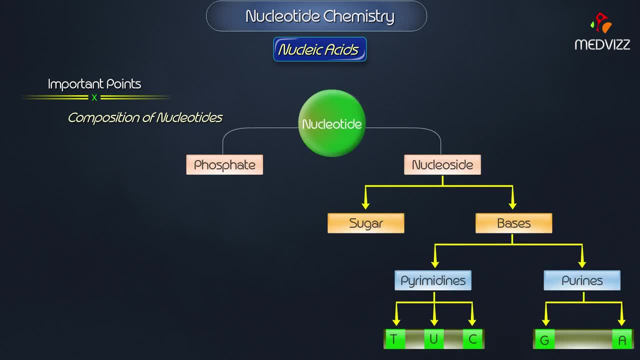 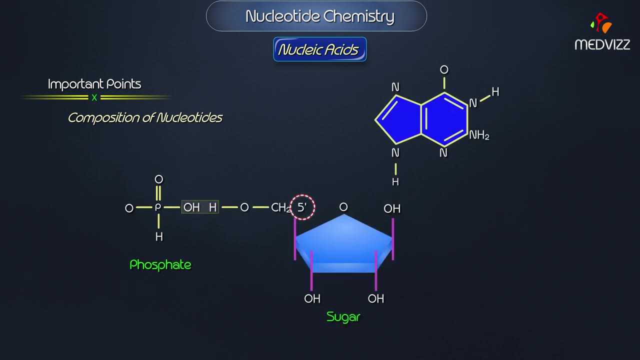 by beta-N-glycosidic linkage. Nucleosides are N-glycosides. Composition of nucleotides: They are made up of nucleoside plus phosphoryl groups. Usually, phosphoryl group is attached to 5-hydroxycline. 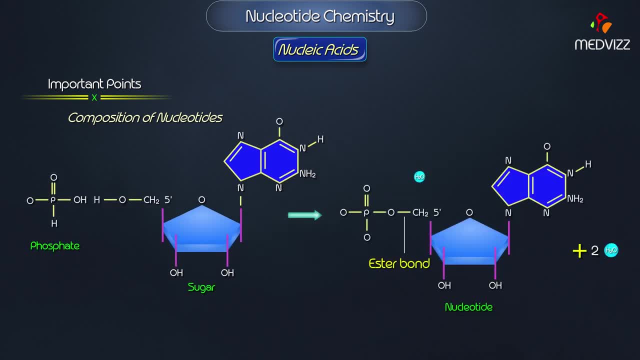 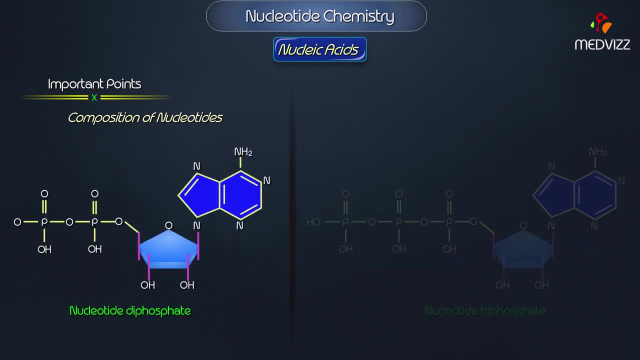 Phosphoryl group is attached to 5-hydroxyl group of pentose sugar by an ester bond. Additional phosphoryl group are attached by an acid-anhydride bond to form nucleoside diphosphates and triphosphates.